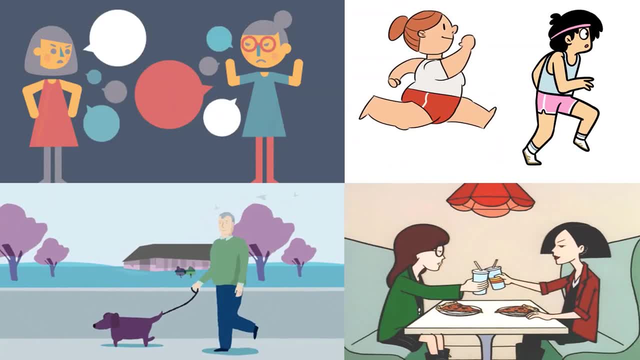 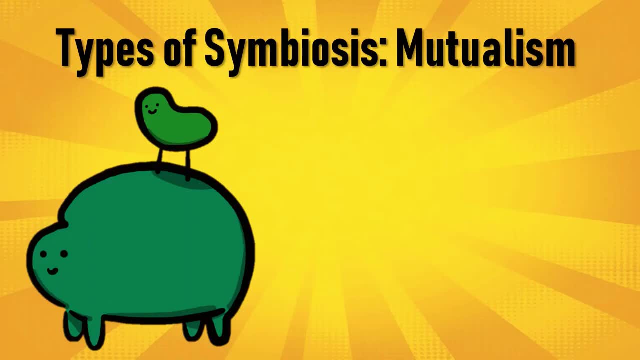 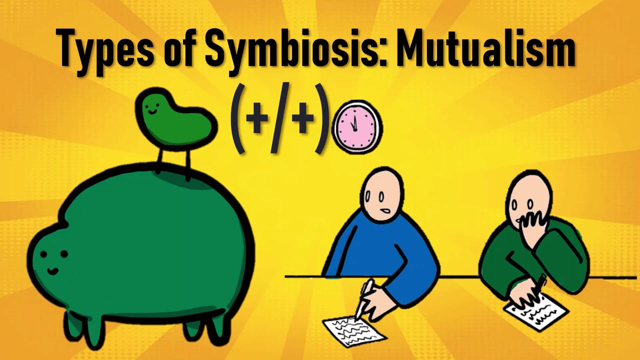 Similarly, when two different species come in contact with each other, there are many possible types of interactions that can occur. Mutualism is a type of symbiotic relationship wherein both the species benefit from each other, Just like you and your friend helping each other for an exam, except for the fact that you two belong to the same species. 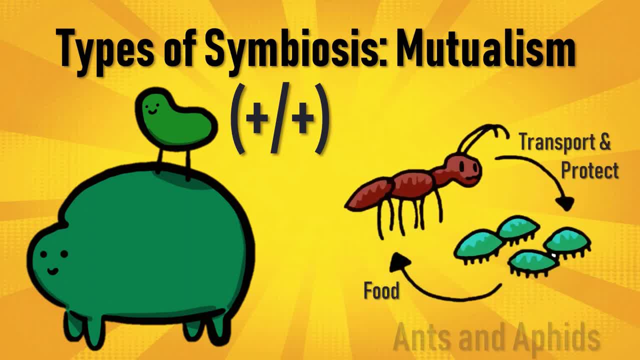 A good example of mutualism is that of ants and aphids, who support each other. Ants can transport aphids to new plants to eat, And they can bring them inside the anthill when it is too cold outside and protect them from predators like ladybugs. 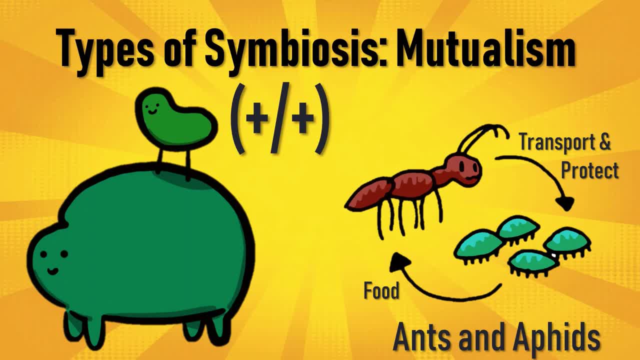 Ants do this because aphid's poop is basically a sugar place called honeydew. Ants take care of aphids, protect them and protect them. Ants do this because aphid's poop is basically a sugar place called honeydew. 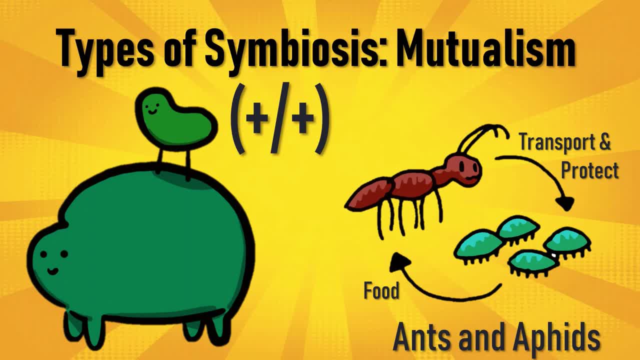 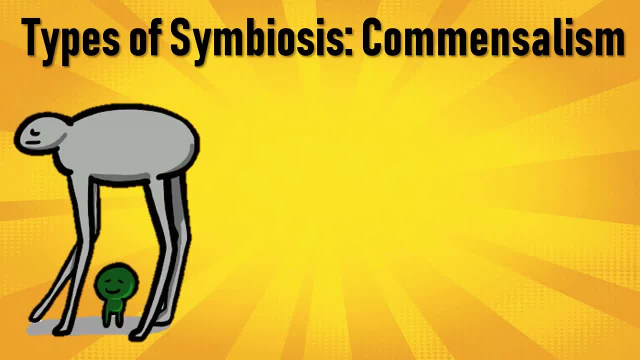 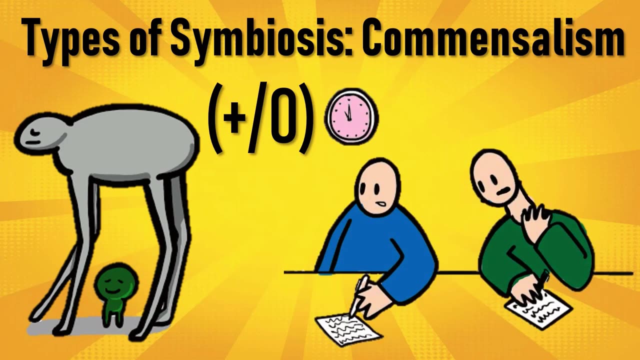 This is called as mutualism. Commensalism is a type of symbiotic relationship wherein one species benefits, whereas the other remains unaffected. It's like your friend peeping into your answers, which won't affect your performance in exams, but it will definitely benefit your friend. 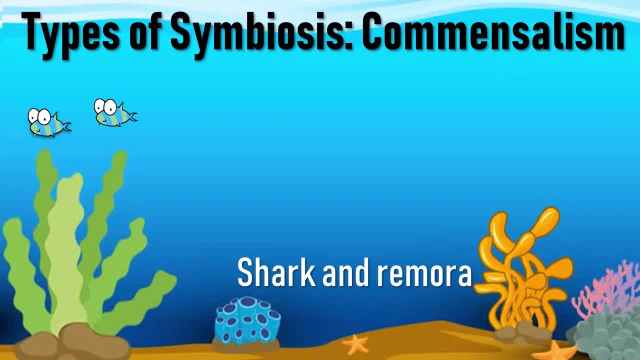 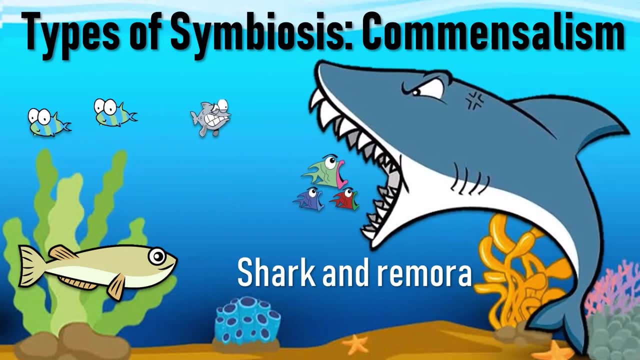 A good example of commensalism is that of a shark and remora fish. When the shark feeds on small fishes, it might leave leftovers which is consumed by the remora fish. The shark is unaffected by this, however, the remora fish is benefited. 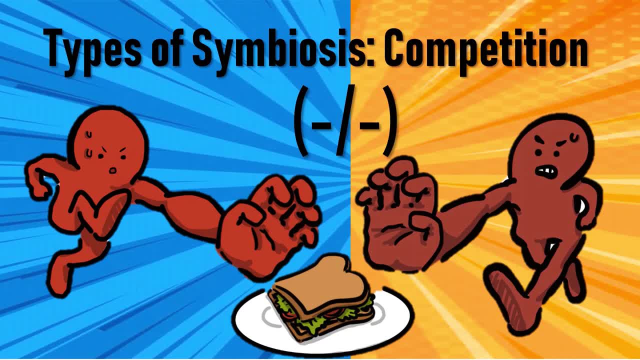 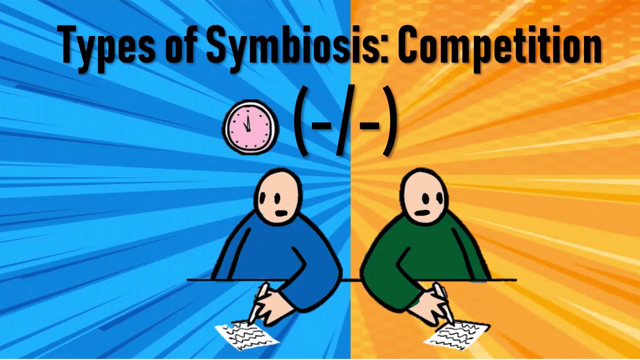 Competition is a relationship between two organisms that has negative effect on both the animals. This can happen when two animals are competing for food, land or for a mate. It's just like you writing your exam seriously to score more than the competitor in class.